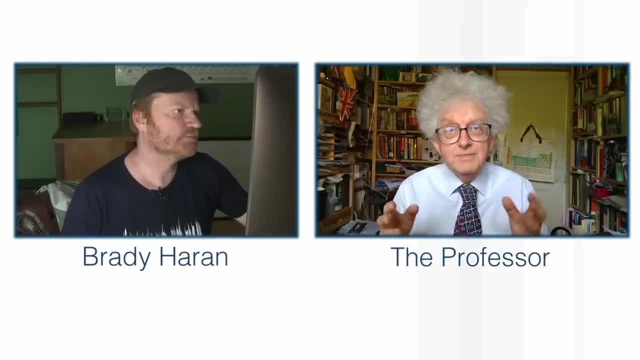 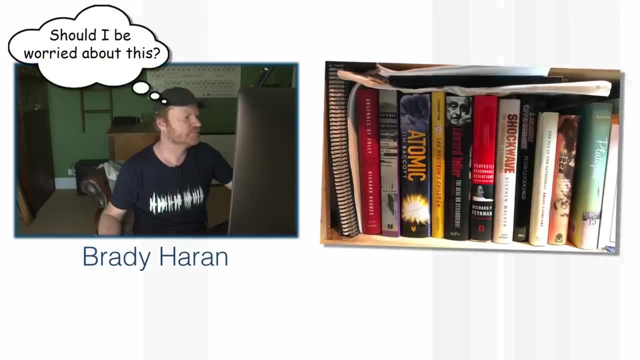 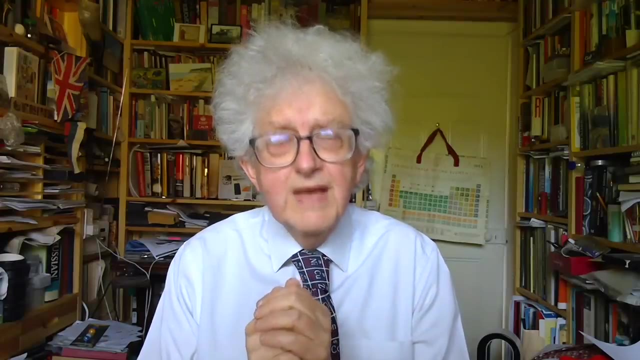 atom bombs. This came as quite a surprise to me because if you look at the shelves behind me, there are quite a few books on atom bombs, mostly on the history, but I never realized that gallium was important and it's only important in the bombs that contain plutonium, such as the one 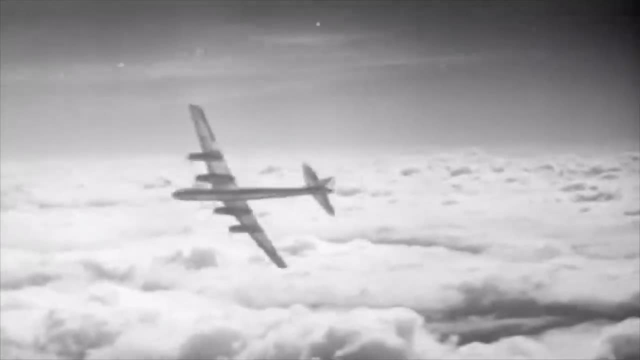 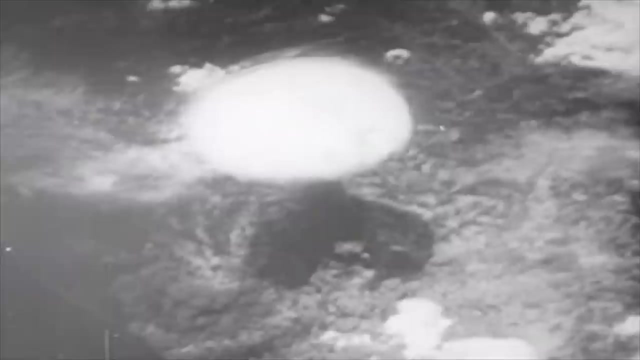 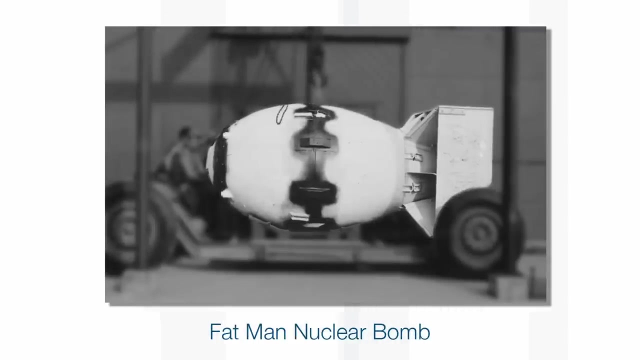 called Fat Man, that was tragically dropped on the city of Nagasaki At 10: 58 the morning of August 9th. the bomb was exploded above the city and in the towering mushroom, Japan could read its doom, And the problem is related to the way that atom bombs work And the way that an atom bomb works. is that one atom of plutonium is hit by a neutron, it splits into two, releasing energy, and it produces two neutrons, each of which go on to react or to split other atoms of plutonium. So you get a chain and the explosion just builds up and up and up. 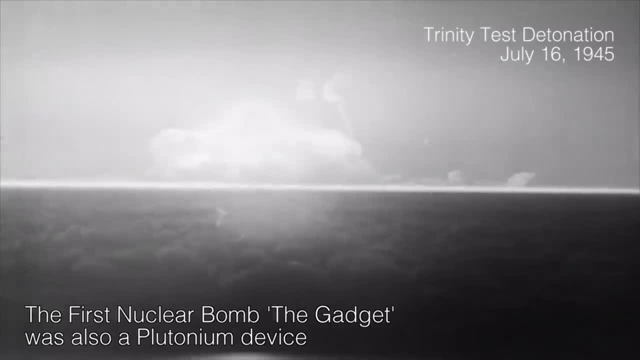 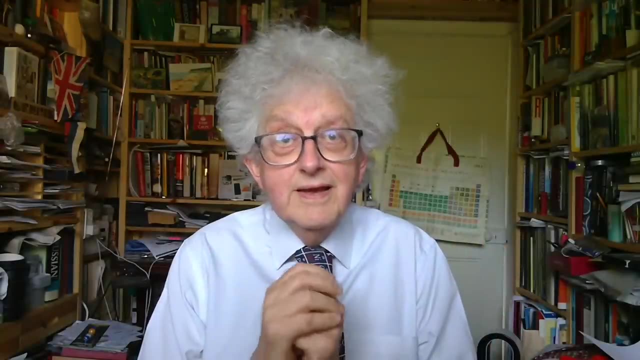 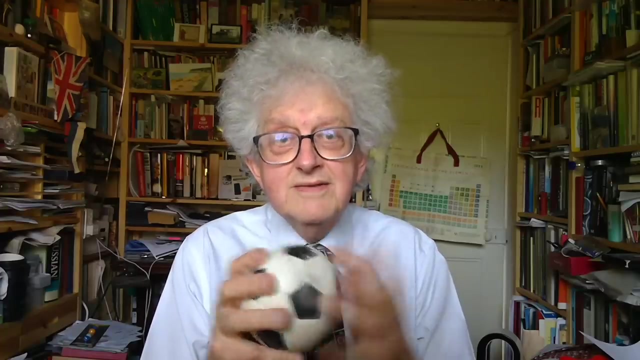 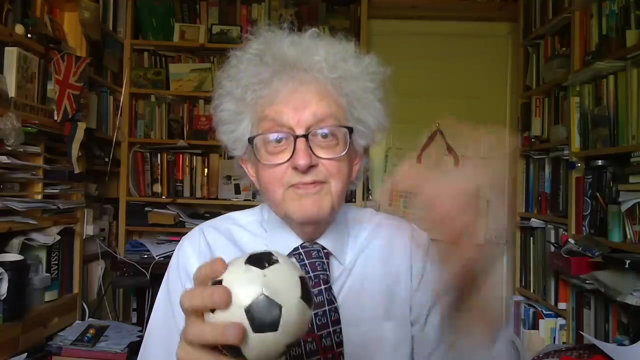 Now there are two problems that you have if you're building an atom bomb. The first one is that you have to have enough plutonium so that if a neutron comes out of the first plutonium atom, it will hit another plutonium atom before it escapes from your lump of plutonium. 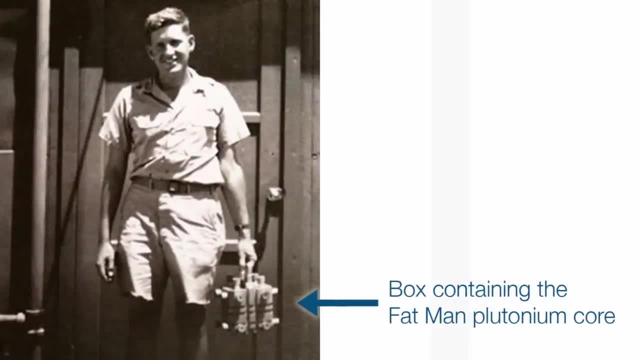 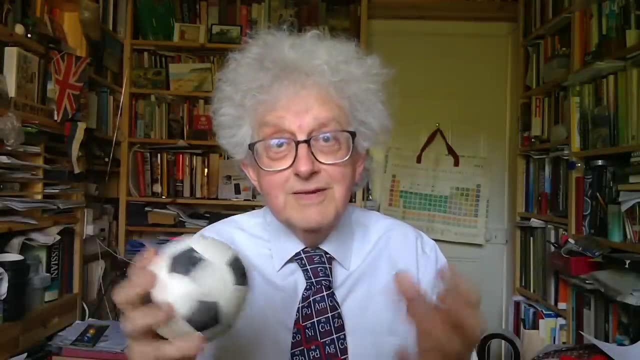 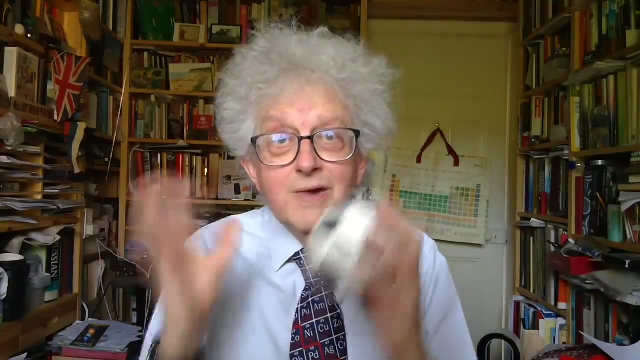 The second problem is you mustn't have too much plutonium or the spontaneous radioactive decay could start the bomb exploding before you're ready. So you have to have a very precise mass of plutonium And one of the ways that they get around this, or they got around this when 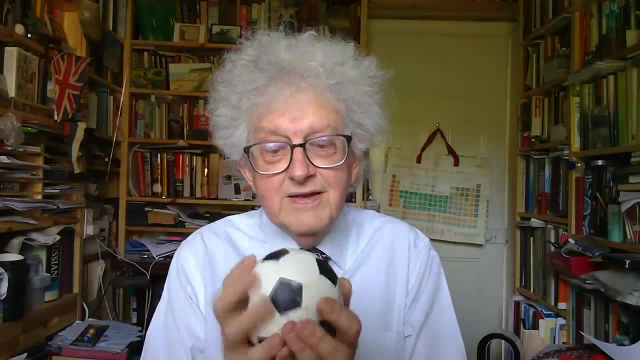 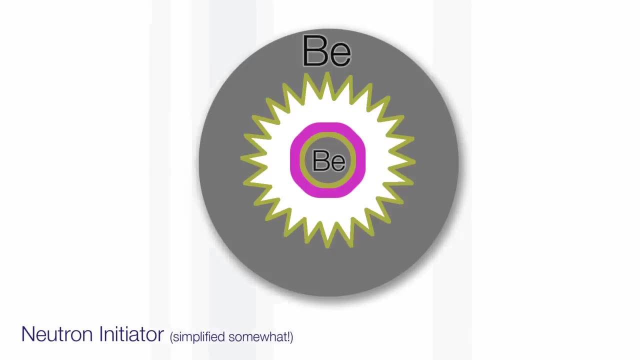 they were devising this bomb was to have a sphere of plutonium which had in the middle two elements, beryllium and polonium, which when you mix them together gives you lots of neutrons. But the beryllium and polonium were separate in the middle And the idea was that the whole of 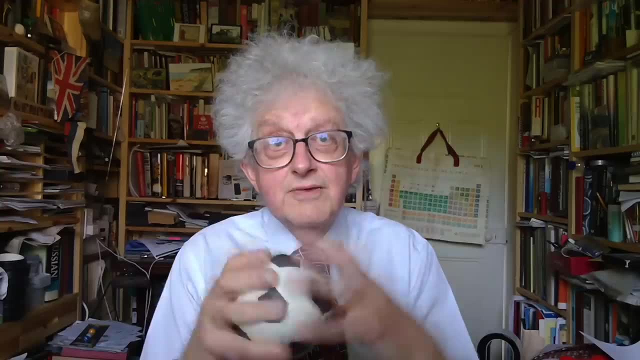 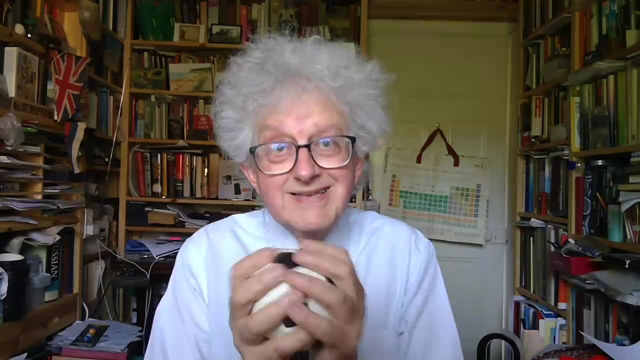 the plutonium was surrounded by explosives. At the right moment all of the explosive would go off and the ball of plutonium would be compressed. It would get denser, The plutonium atoms closer together, so it was harder for the neutron to engage. So we had a ball of plutonium and atta. 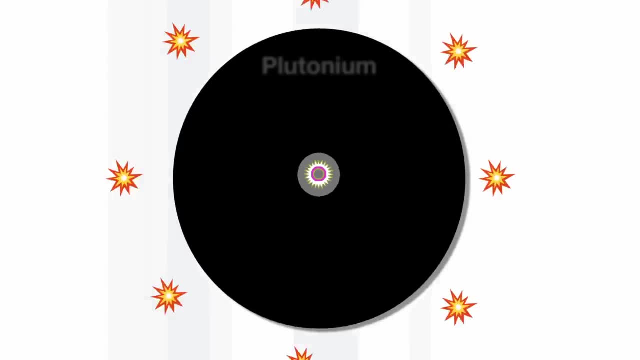 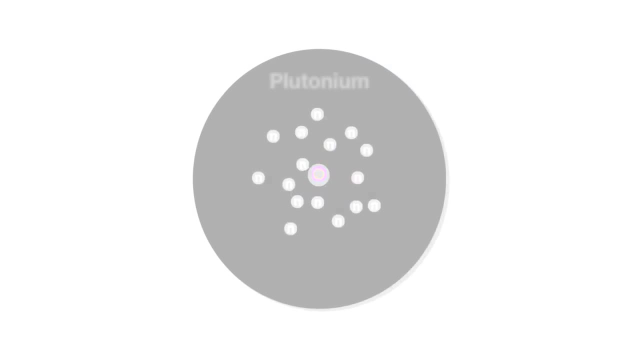 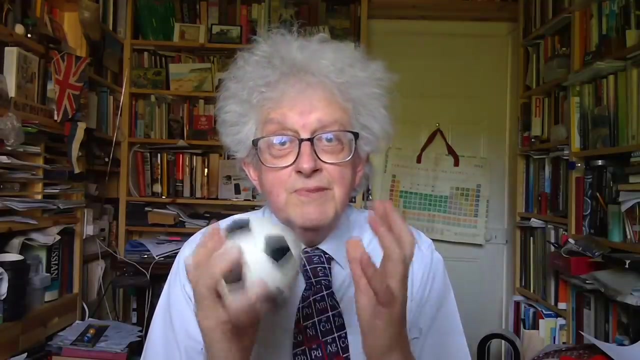 the neutrons to escape, and at the same moment, the beryllium and polonium would be mixed up together and a big number of neutrons would be released. to set the thing off, Now, the key point was that the sphere of plutonium had to be absolutely. round, because otherwise when you tried to compress it, if it wasn't round it would squash into the wrong shape and wouldn't get dense. And the difficulty is that pure plutonium is very difficult to make into a shape. The technique they used was called hot pressing, so that you take heated mould and press it at. I think. 400 degrees centigrade With pure plutonium, you get the so-called alpha phase which, when you press it down, you get the so-called alpha phase which, when you press it down, you get the so-called alpha phase which, when you 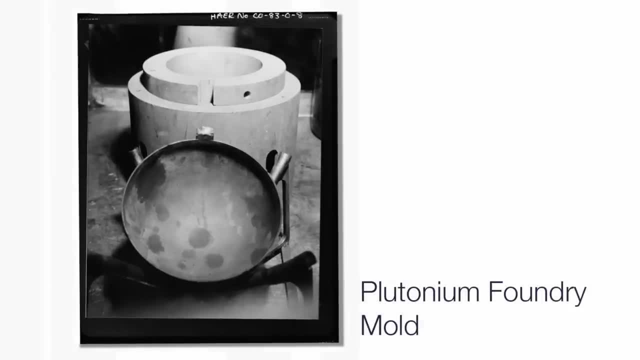 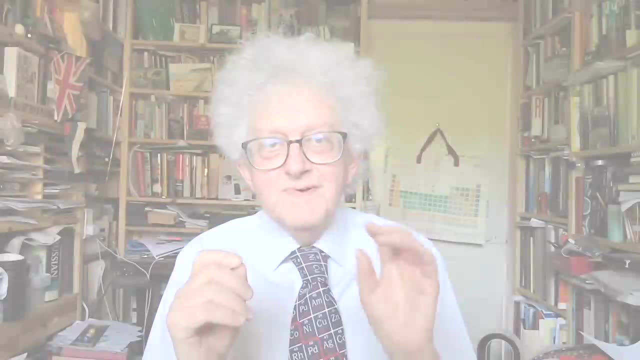 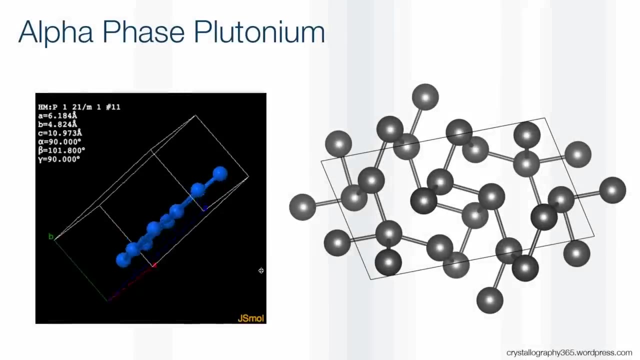 take the mould apart, begins to flake off and is not suitable. It was realised that you could mix the plutonium with a small amount of another element which would change the arrangement of the atoms in the metal, so-called different phase, instead of the alpha phase, so-called delta phase, which was 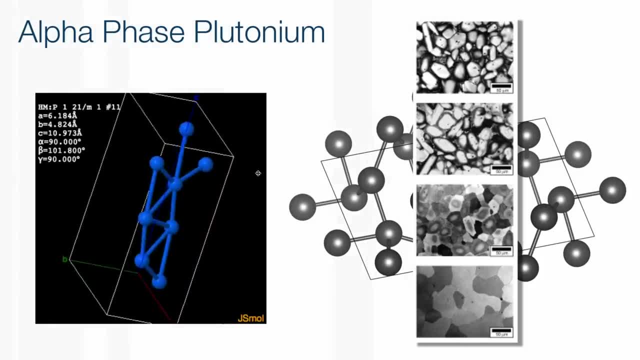 slightly less dense and much easier to mould or to hot press. They began by trying to make the plutonium as dense as possible. They began by trying to make the plutonium as dense as possible. They began by trying to make the plutonium as 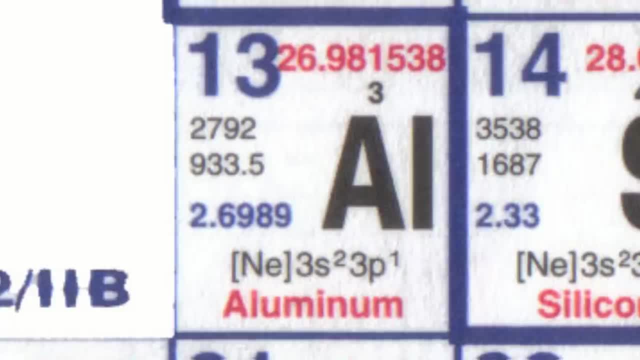 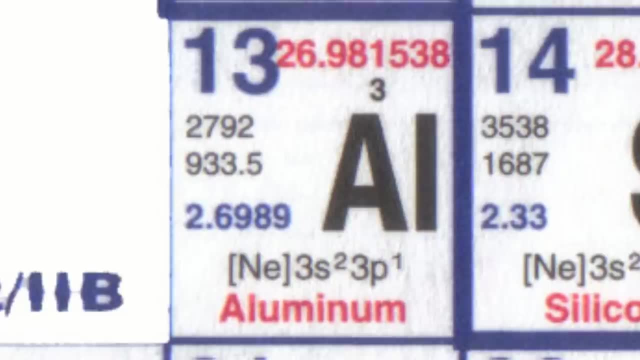 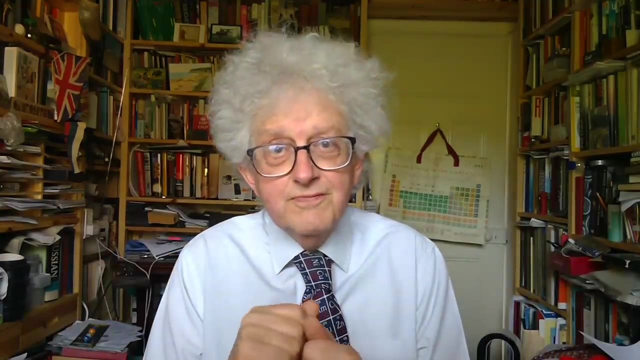 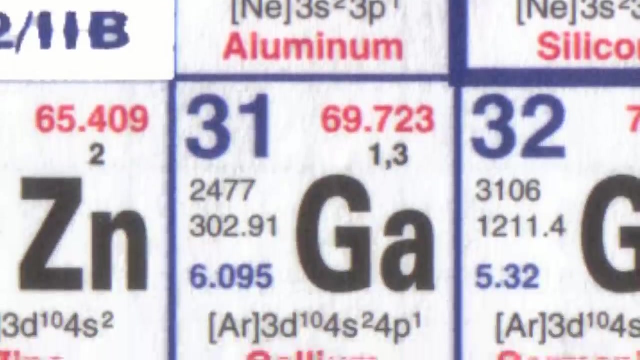 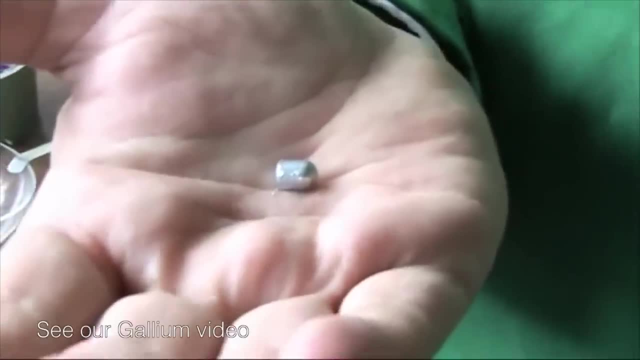 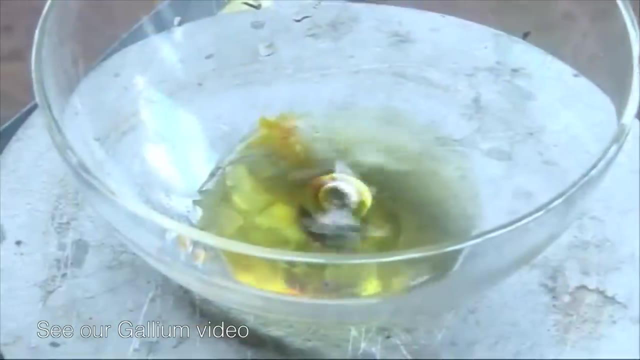 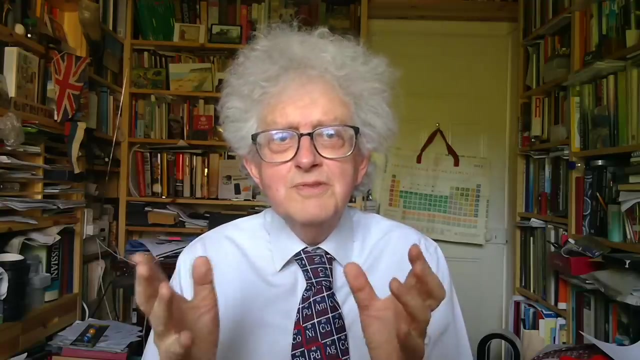 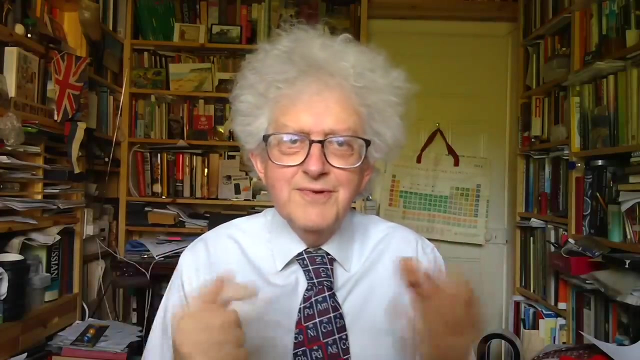 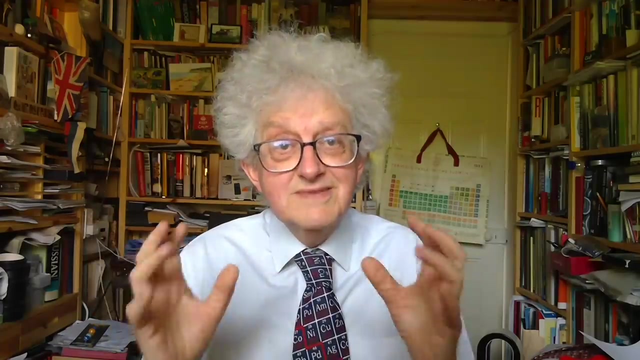 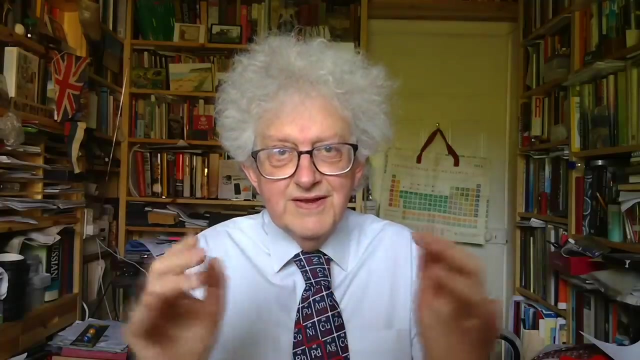 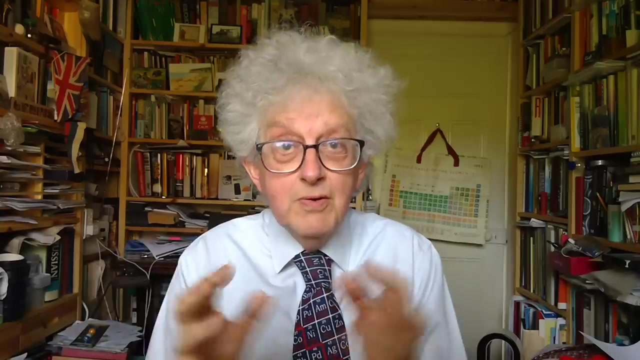 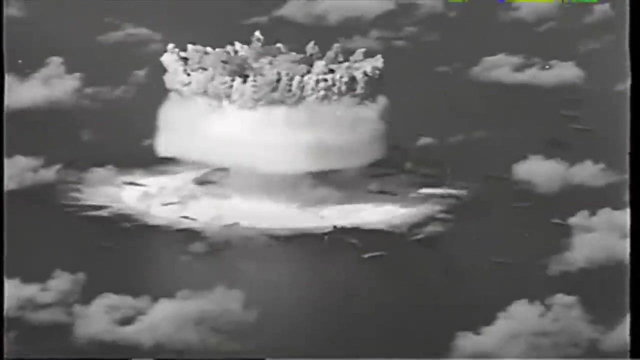 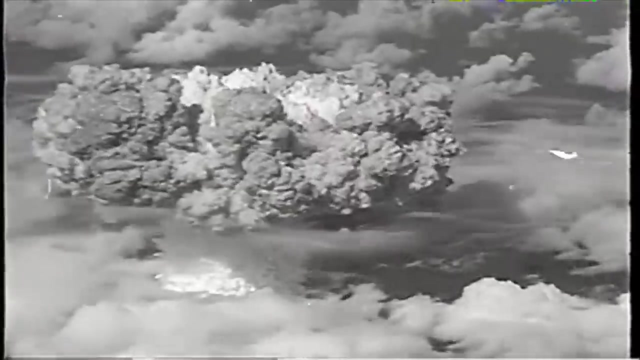 plutonium as dense as possible. They began by trying to make the plutonium as dense as possible. They began by trying to make the plutonium as dense as possible. They began by trying to make the plutonium as dense as possible. They began by trying to 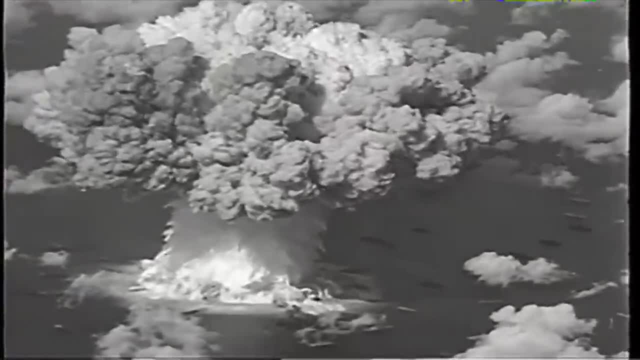 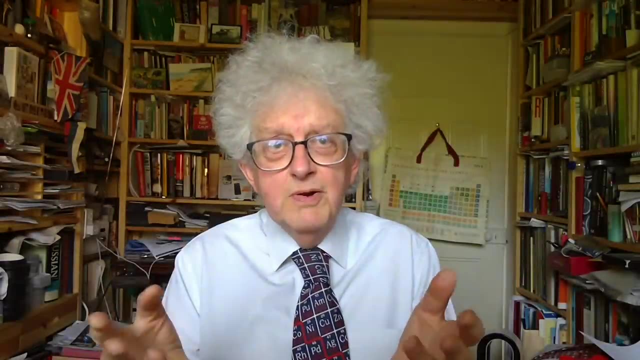 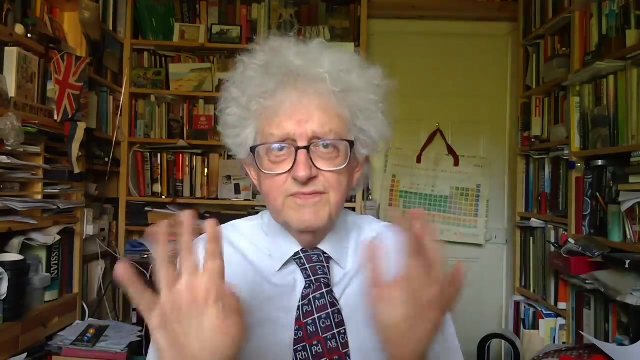 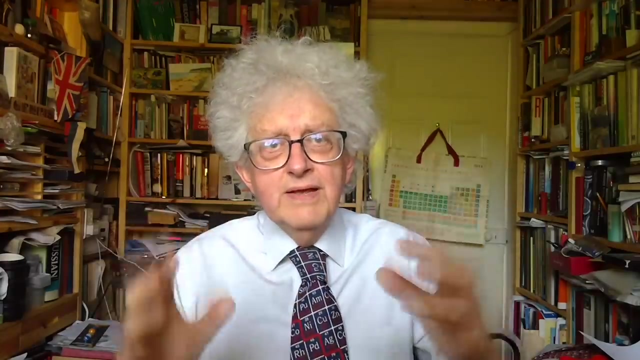 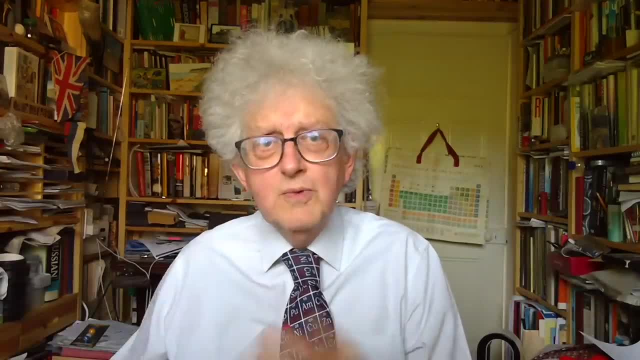 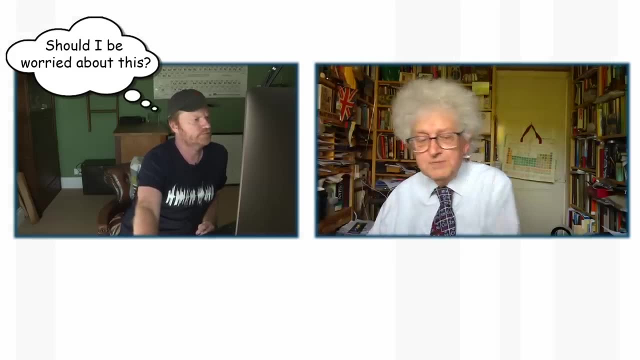 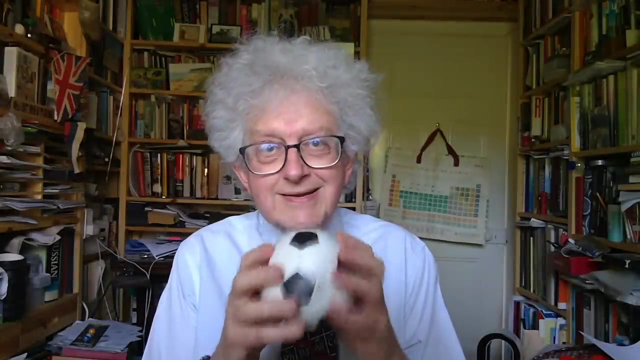 to put the whole thing together, One of the books that I've got called Atom Bombs has quite a nice picture inside showing how this is put together. But the reason for having this ball is this ball is almost exactly the size: 3.62 inches in diameter. 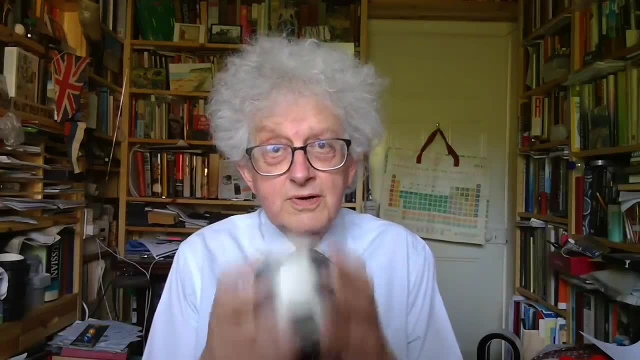 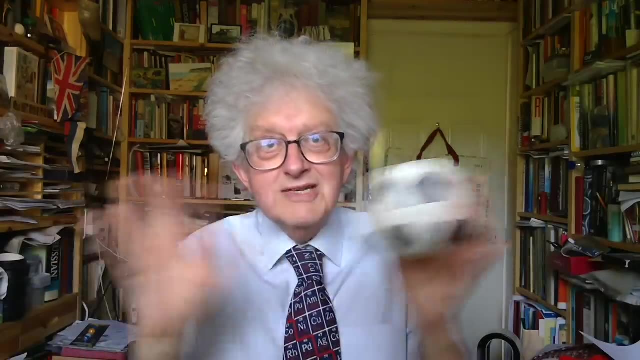 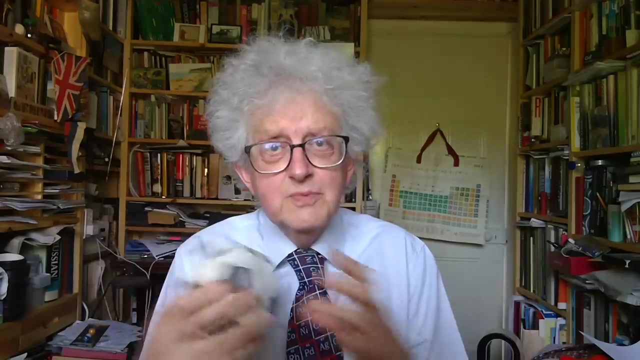 9.2 centimeters of the core of the Fat Man bomb, So it's really not very big. and when the bomb actually went off, the amount of plutonium that split and gave the energy was only one gram. The ball of plutonium weighed over six kilos. 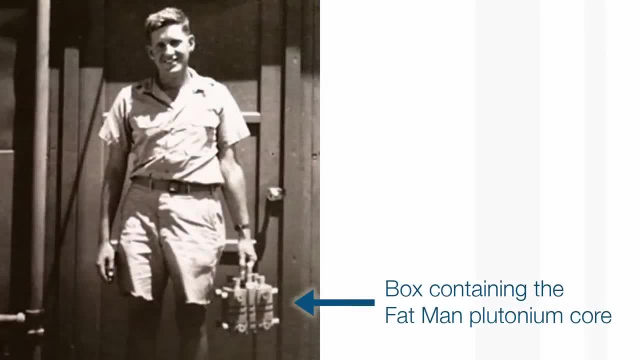 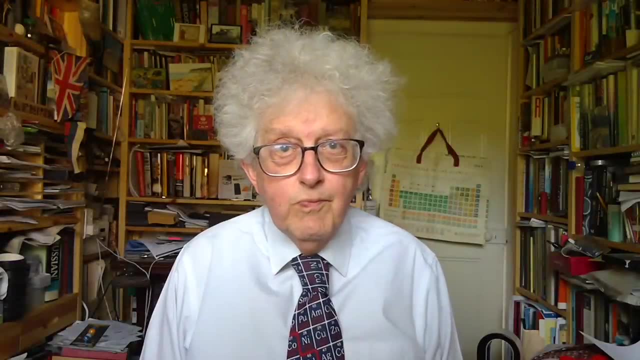 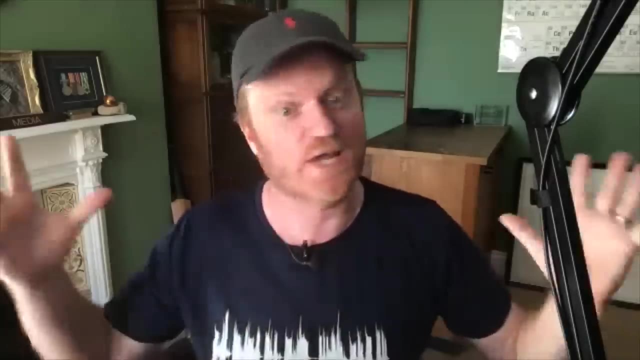 so just a tiny fraction of that actually caused the explosion and presumably the rest of the plutonium was blown all over the place. The gallium was an important ingredient, but it was an important ingredient for the manufacturing of the ball, not for any part of the detonation or explosion or anything. 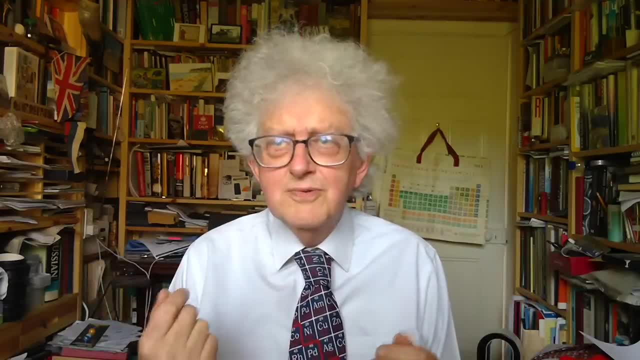 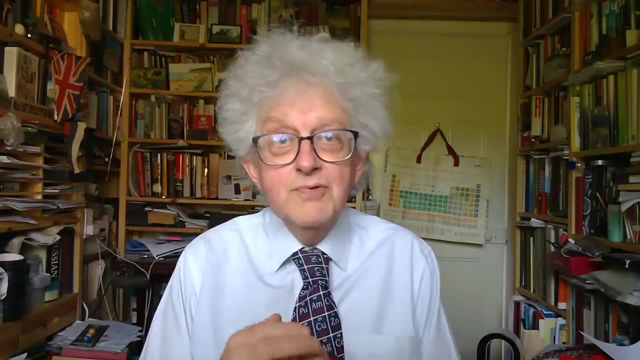 And according to a website I looked at called FAQs about nuclear weapons, gallium is still used for making modern nuclear weapons. Professor, do you think all these books you're buying and websites you're looking at are going to get you on some kind of watch list? 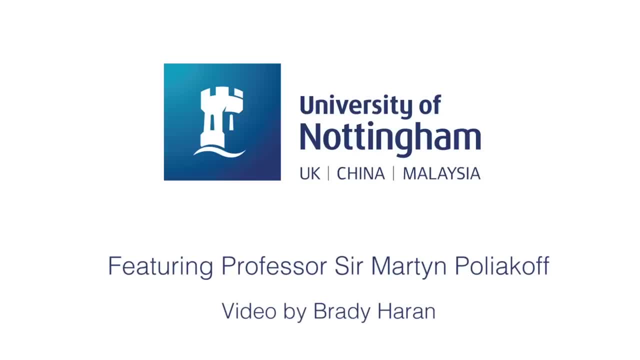 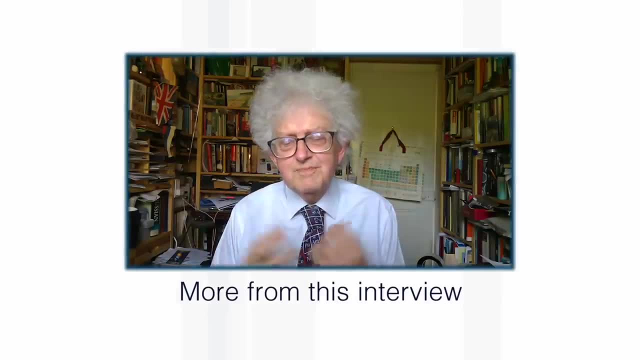 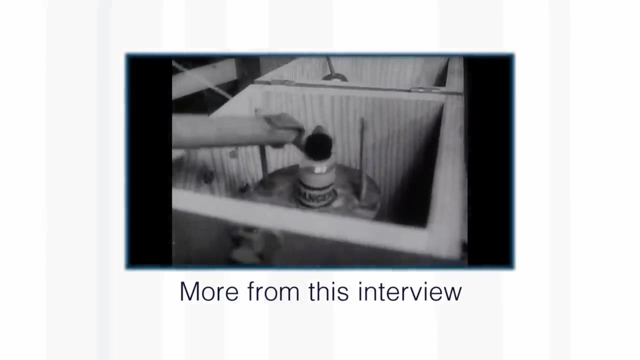 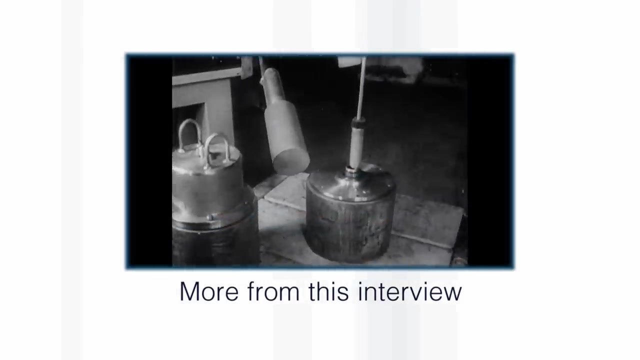 Oh, I hope not, But I think that the history of the project of the atom bomb is extremely interesting, not only for the physics and the chemistry that was involved, but the deep moral question that has always worried me, that if I had been a scientist during the Second World War?